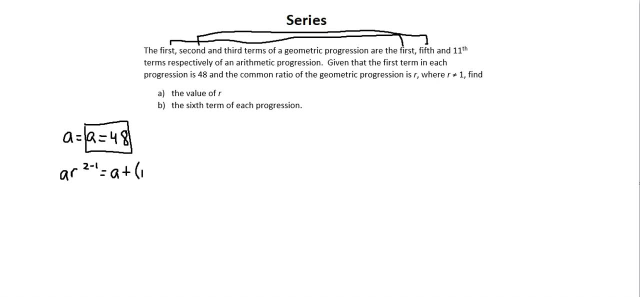 is a plus quantity, n minus 1 times d. Here my n is going to become 5, and I can simplify this equation to a. r equals a plus 4 d, And the third equation, the third term of the geometric, goes with the eleventh term. 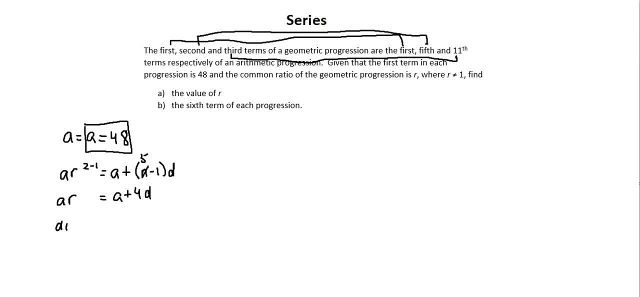 of the arithmetic. So we will have: a r to the power of 3 minus 1 equals a plus quantity 11 minus 1 d. Here, simplifying to a r squared equals a plus quantity 11 minus 1 d. Now of the two remaining equations with unknowns for my r, looking at requirement a, the value. 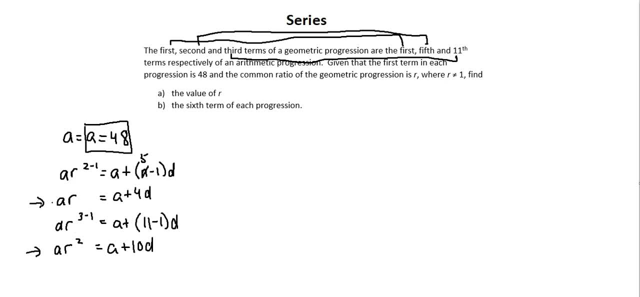 of r in the first equation. there I've pointed out with the arrow I have r to the power of 1.. That's easier to work with than the r to the power of 2 in the second equation. So I'm going to come up here working with this equation. 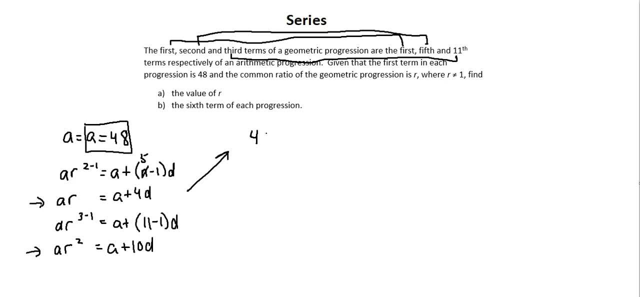 The a I know is 48.. So I'll replace the a's with 48.. So 48 r equals a, plus becomes 48 plus 4 d. And now to solve for r, I'll divide both sides by 48.. Dividing by 48.. 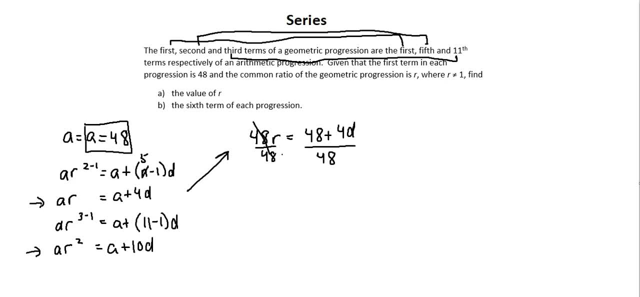 And r equals 48 plus 4 d over 48.. Now into my second equation. I need to use a different equation now. the substitute in my r value a times r squared- Again I know a- is 48 times r squared. 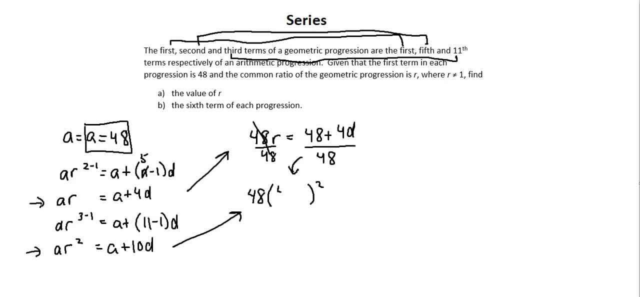 My r value is what I've just simplified to The fraction 48 plus 4 d over 48.. So I have on the left: ar squared becomes 48 times 48. Dividing by 48.. 48 plus 4d over 48 squared equals a plus 10d, is 48 plus 10d. 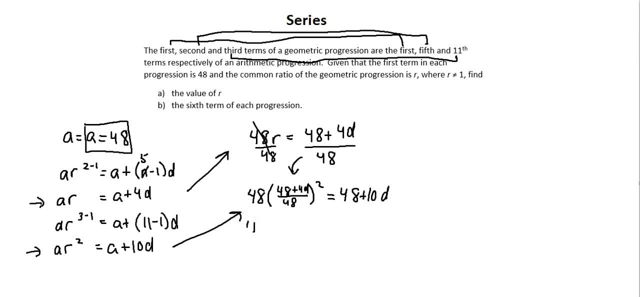 Working through some algebra, we're going to end up with 48 times quantity, 48 plus 4d squared. divided by 48 squared, the 48 in the denominator of the fraction that is being squared is 48 squared. I'm going to write that as 48 times 48, and now I'll eliminate 48 from the numerator and from. 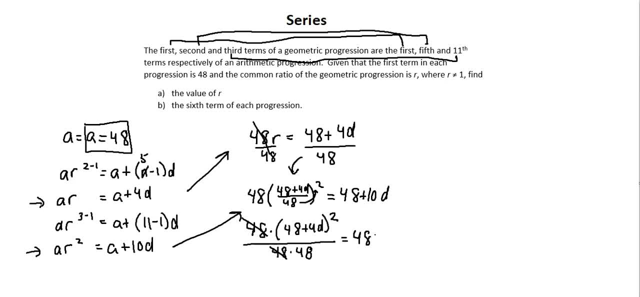 the denominator equals 48 plus 10d. Now I will multiply both On the left: when I multiply by 48, that offsets with the denominator 48, and now I'm left with 48 plus 4d. squared equals 48 times 48 plus 10d. 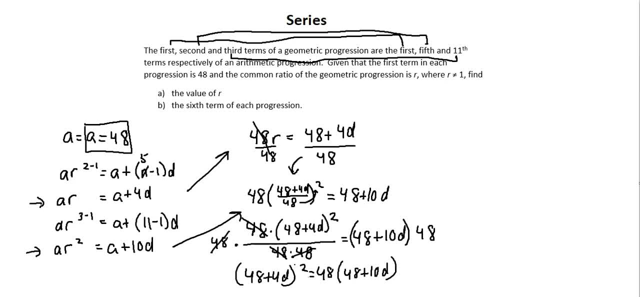 Now you might recognize that, because on the left I'm multiplying by 48, I'm going to end up with 48 squared. On the left I'm squaring an expression that involves the variable d. This is going to end up as a quadratic. 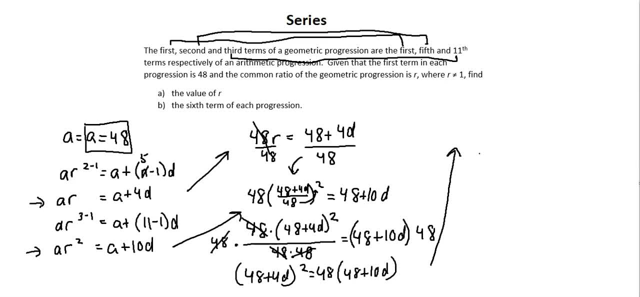 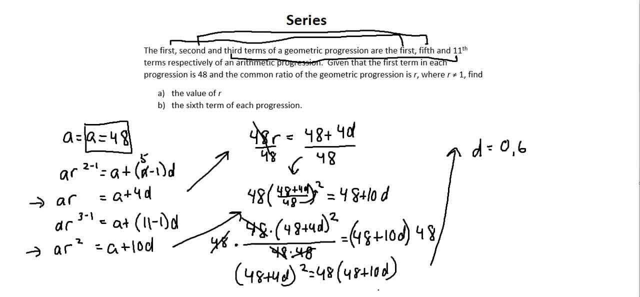 Let's then calculate the value singular of r. So there's a clue formula. Let's see what happens when I calculate my two r values. The way I'm going to calculate r: r equals. looking at the top of center column: r equals. 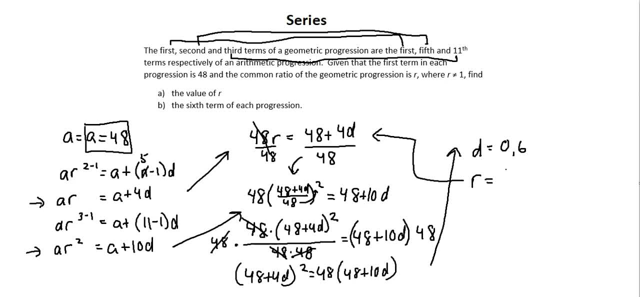 48 plus 4d over 48.. The way I'm going to calculate it is to do a approximation that will depend on how many interests there are. equals 6 case. So r equals 48 plus 4 times something over 48.. Again, r equals 48 plus. 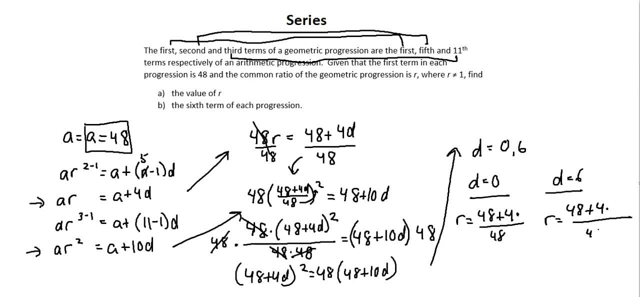 4 times something over 48.. On the left, the d is 0,, so I have 4 times 0.. On the right, the d is 6,, so I have 4 times 6.. When I complete both of these calculations, I'll end up with r. 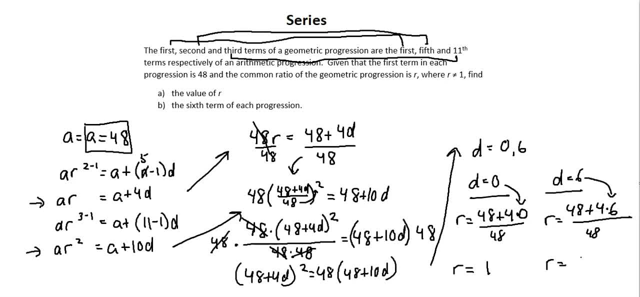 equals 1 and r equals 3 over 2.. Notice in the requirements that the r value r does not equal 1.. Therefore I disregard the solution producing r equals 1, and I've now answered requirement 2.. Requirement A: the value of r equals 3 over 2.. Now requirement B: the sixth term of each. 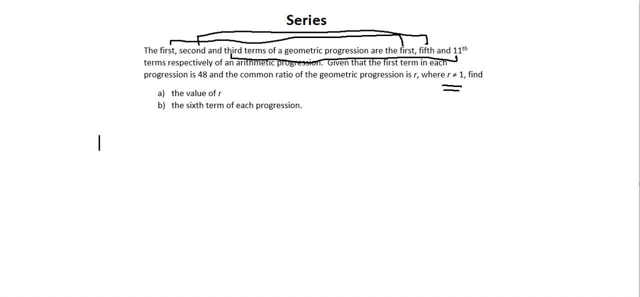 progression For requirement B: the geometric series, sixth term, and the arithmetic series, sixth term. For the geometric term we have 48, which is A times r. We've calculated as 3 over 2.. 3 over 2 to the power of sixth term is an exponent of: 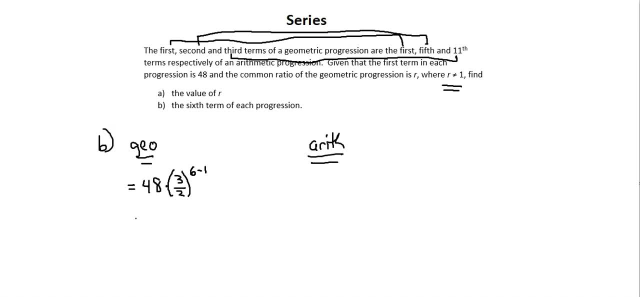 6 minus 1.. So 48 times 3 over 2 to the power of 5 simplifies to 729 over 2.. And in the case of the arithmetic sixth term, we have 48.. The dimensioned dimension of r is the values of the two values d and 6.. 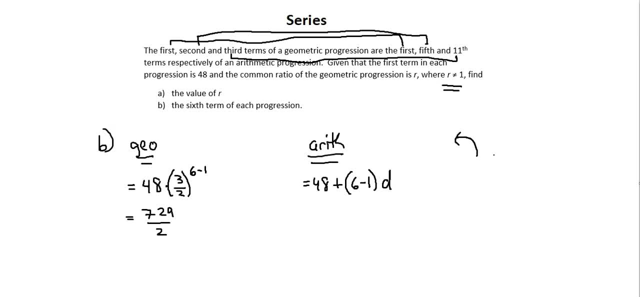 For D. we have a value of a value d, So we have 0 and 6.. This equation should be in the form of the first value of r. We need a value for r. we need a value for d. We already know that r equals 2.. This Euh eqable. r equals 3 over 2.. As always, what? 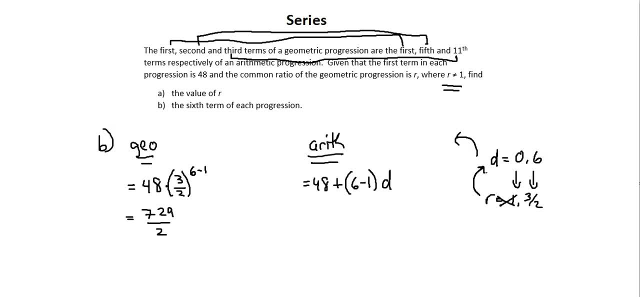 we can do is to work with r. For r we need about 2 values of d, We need about 2 values can't be 1.. So the d that led to the value of r we can't use. we can't use d is 6.. So continuing.